In the power term, which is that is associate with Power distribution, is a key point of knowledge about power electronics, Power dispersion, which is aеr the back失aint aspect of power electronics, Heat transmission, which is what we are dealing to focus about. In power electronics, usually we are dealing to have high power generation, transmission and distribution, which is what we are dealing to focus in power term, which is the associated with powerpolKnəR stoRm. power description, which is the associated with power belt and other body parts we are dealing to focus. 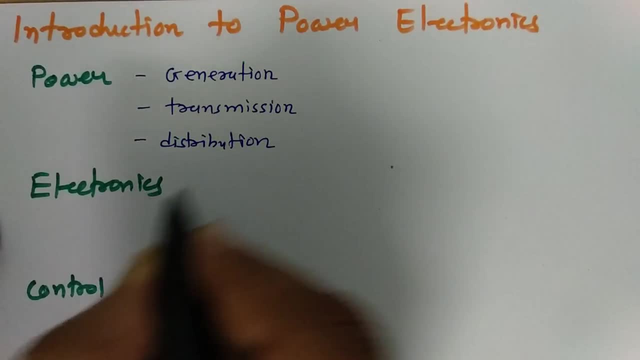 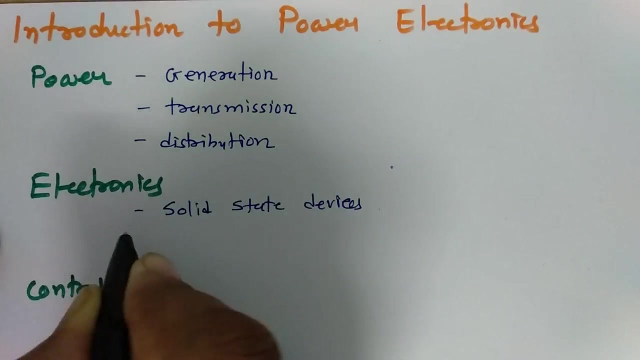 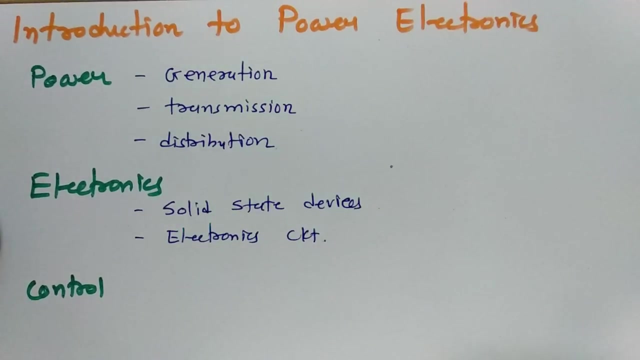 power electronics. Now when we talk about how electronics is associated with power electronics subject, then usually we focus on those solid state device which is functioning at high power. So we study solid state devices which is functioning at high power. in power electronics We study some electronic circuits which is useful to control high power devices and even 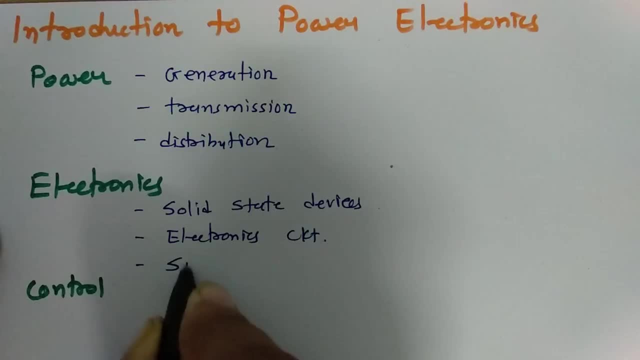 sometime. we need to focus on signal processes Now, here this signal process says that is associated with high power signal process. It is not the signal processing which is there in digital signal processing or adapted signal processing, but here we are dealing with to focus about high power signal processing. 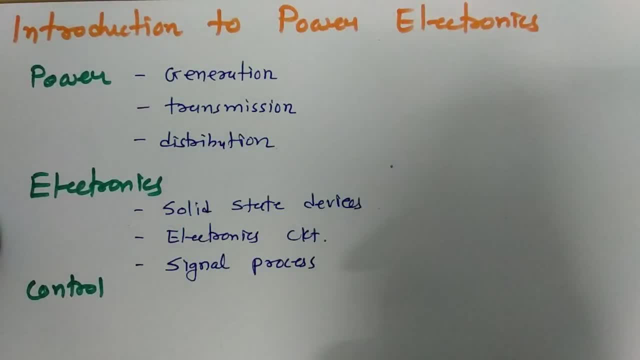 aspects in this electronics term. and at last, when we talk about controlling of high power, we usually study steady state characteristic and dynamic characteristics. So, in terms of controlling of devices at high power, So when we talk about the controlling of high power, However, we will be studying steady state characteristics and dynamic characteristics. 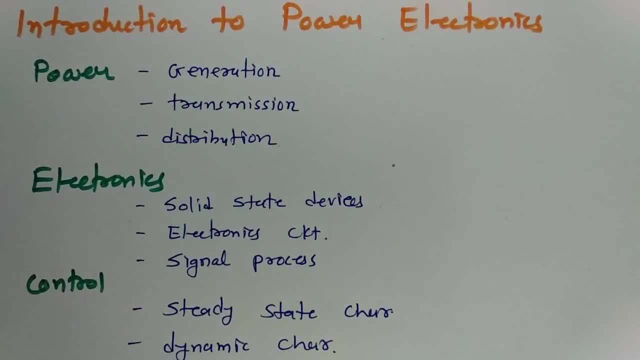 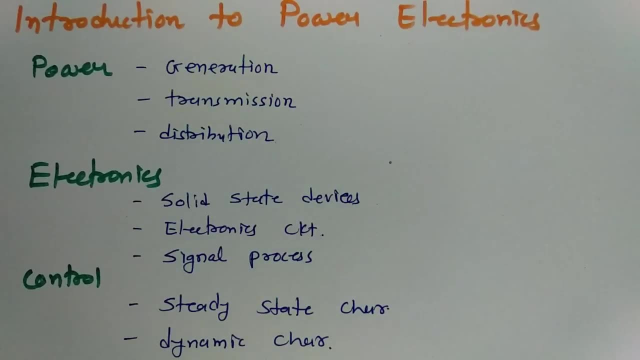 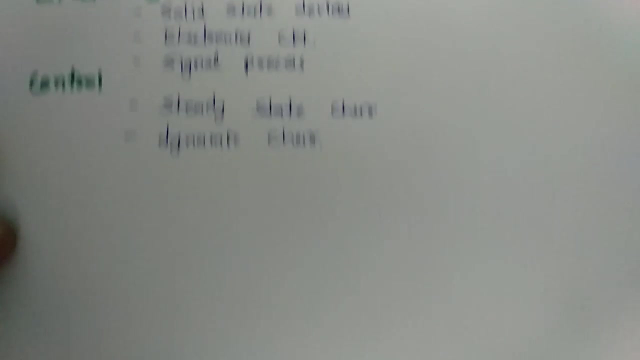 So all those things that I will be going to cover in complete subject of power electronics, which is associated with this playlist. So one who is interested about power electronics understanding in that way, this is what the playlist which is associated with this terminology. Now let us try to understand what we do exactly in power electronics. 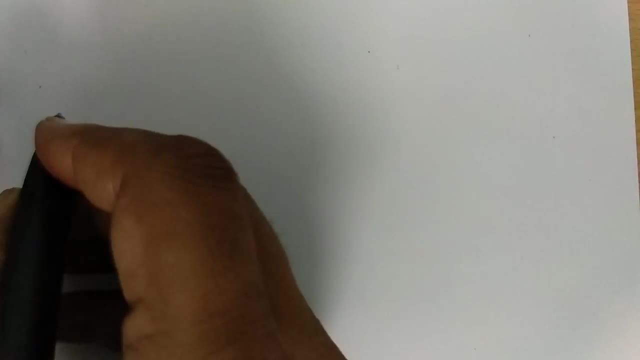 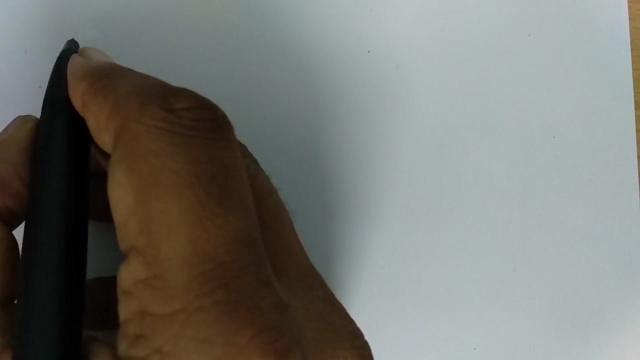 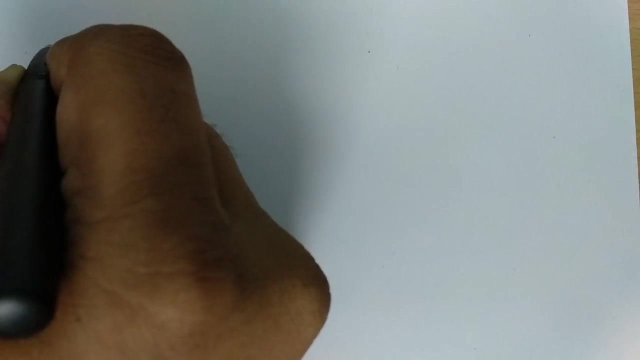 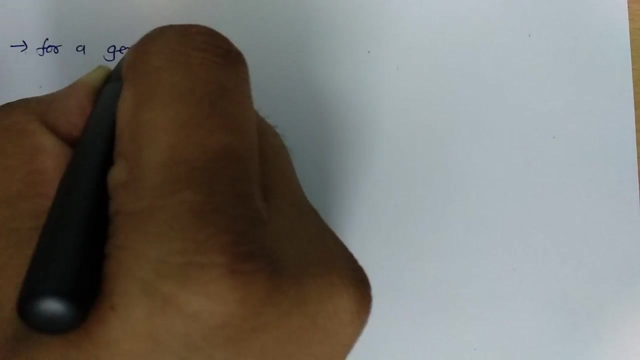 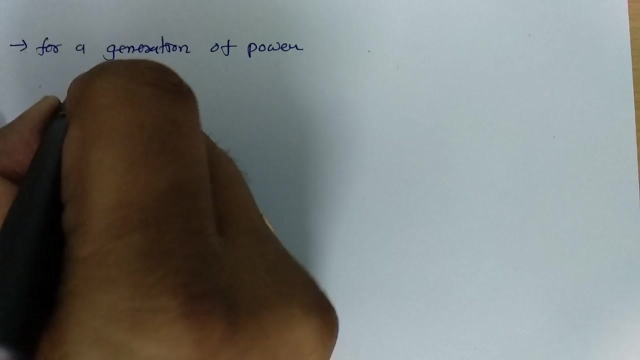 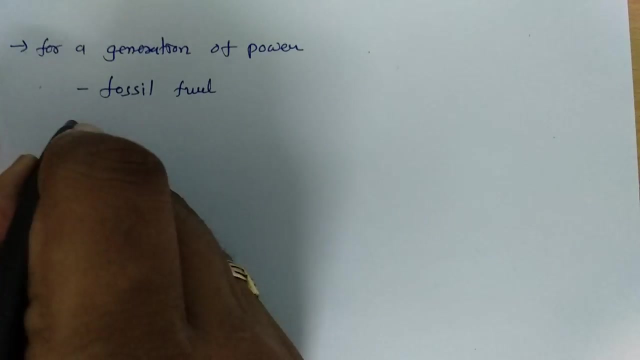 So when I talk about power electronics and when I talk about generation of power, then generation of power that is what we are generating By using fossil fuel or nuclear resources or renewable resources. So for a generation of power We use fossil fuel, We use nuclear. 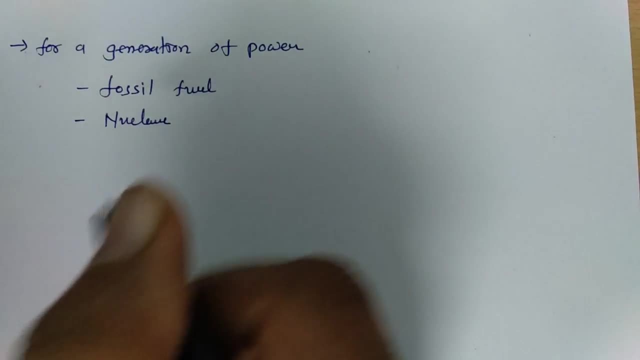 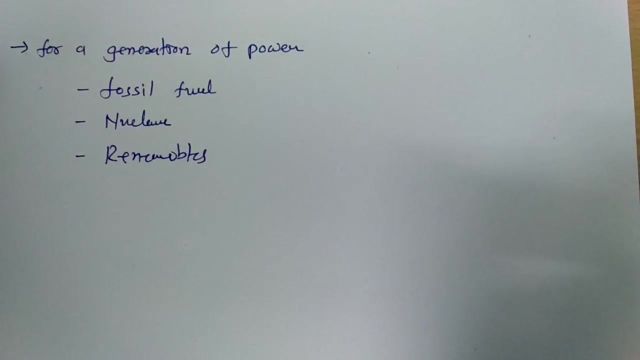 Fuel, and even renewable. That is what we are using it to have a generation of power. Now, what is the basic process? Let us try to understand that and at the end we will be able to conclude. what is the role of power electronics engineer in this complete process? 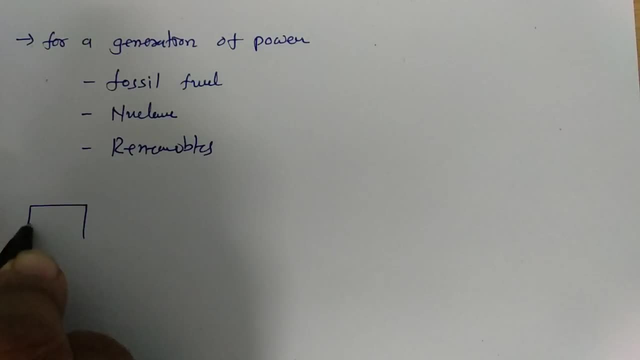 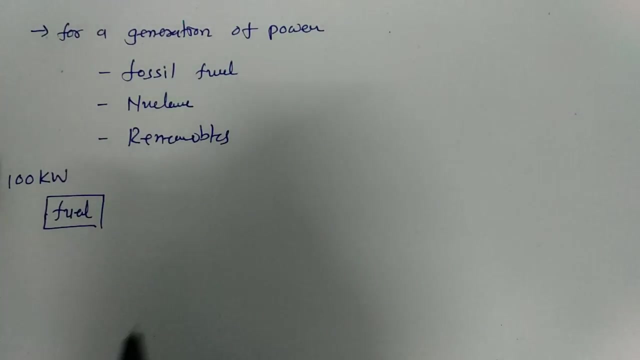 So We have a fuel. Let us say by fuel, I am generating 100 kilowatt of energy. Now, this 100 kilowatt of energy, that is what we are giving it to turbine. Now, when we generate 100 kilowatts of energy and out of that energy, what will happen is this: is what power actually 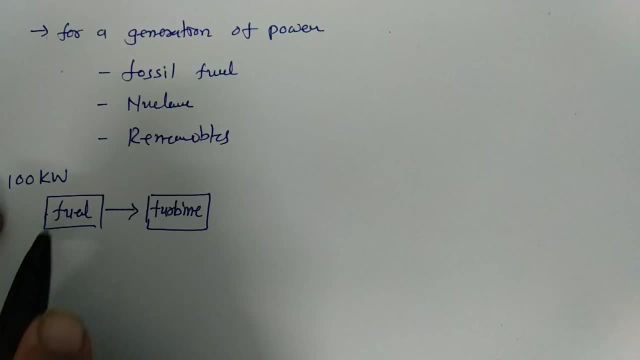 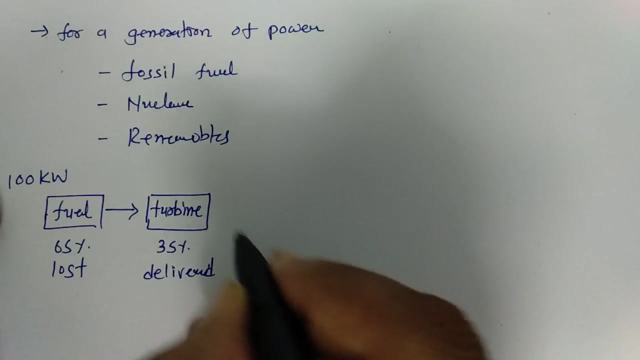 but with respect to time, we are generating it. So, out of this power, 65 percentage power will get lost And only 35 percentage that will get delivered To the turbine. And then, after the power, which is what there with turbine, which is there in terms of mechanical 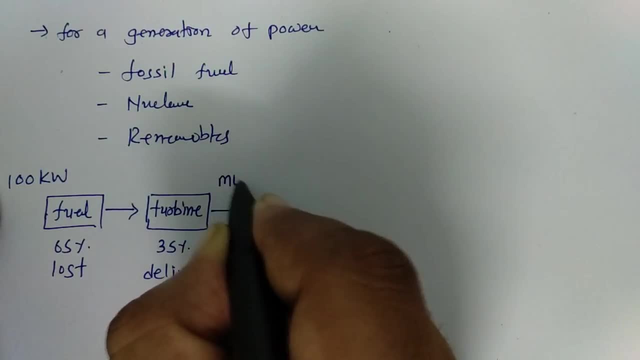 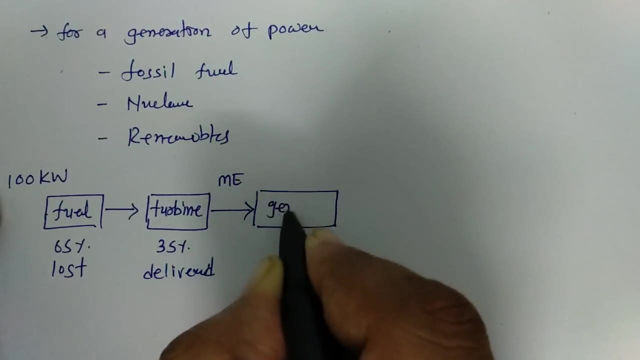 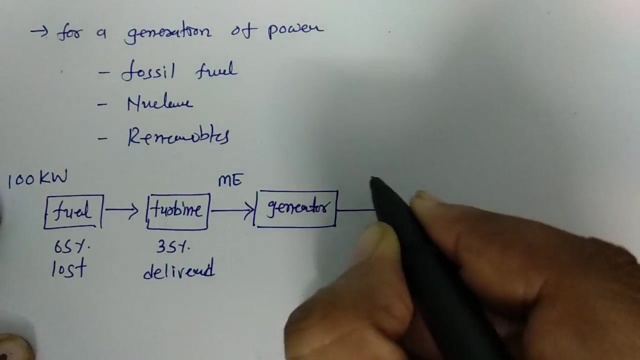 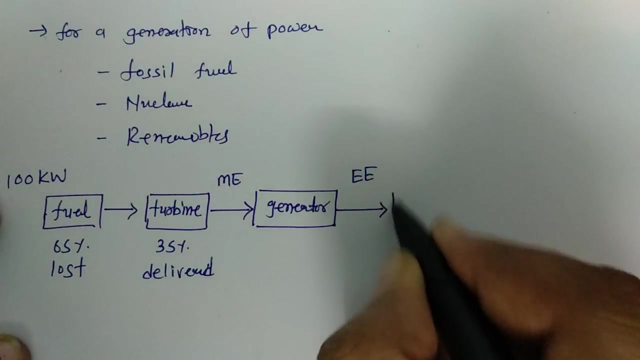 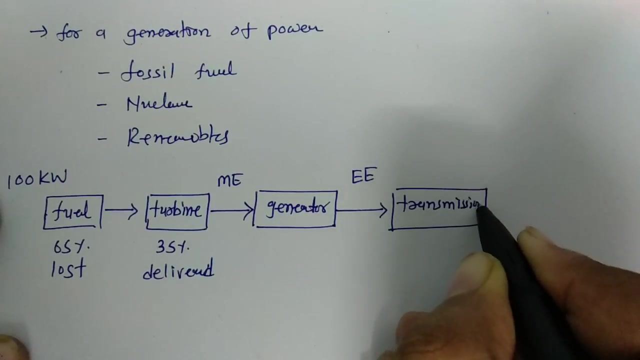 energy. So to have electrical power, I need to have a generator. So I will be connecting generator here. So This generator, This generator, will translate mechanical energy into electrical energy And then, after there will be transmission line, which is what we are using it to transmit. 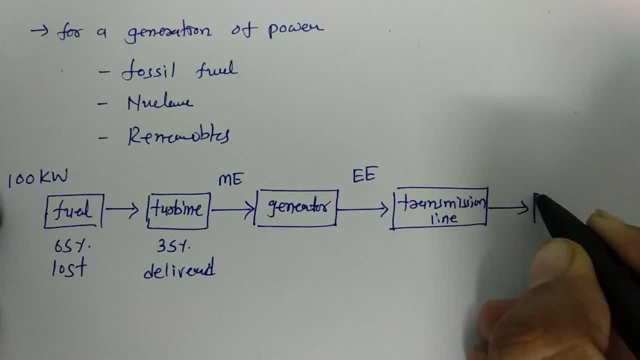 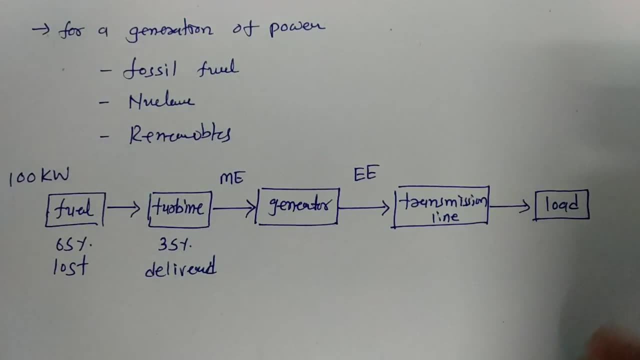 signal to the load, So at the end there will be load. Now, when we see how much power that is getting delivered to the load, So that power delivered to the load that we usually one can identify, it is around 16 percentage. Now, see all those data's, those are approximated data and that is what, even improving with 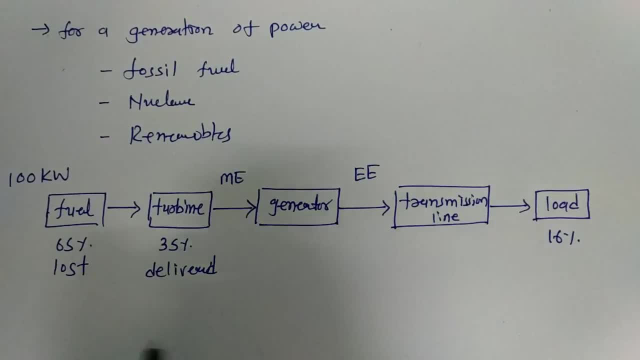 respect to time. the reason is technology is getting improved, So this data that I have took it from some references, which is what even Explained before 5 to 6 years from now I am right now, I am just making this video- in 2018, initiation. 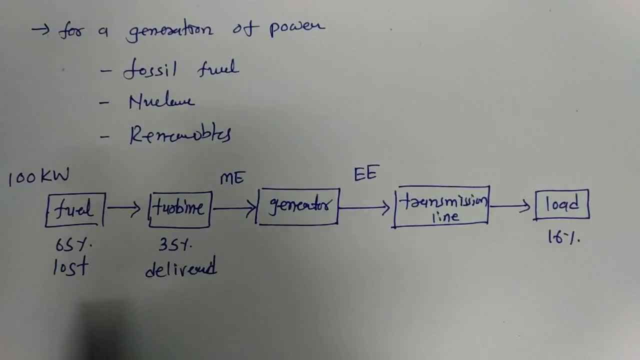 So one can understand, like: see, this is what the data which was there in 2011 or 10 around, But one can understand what is happening exactly. We are using fuel And that is what Generating power of 100 kilowatt. 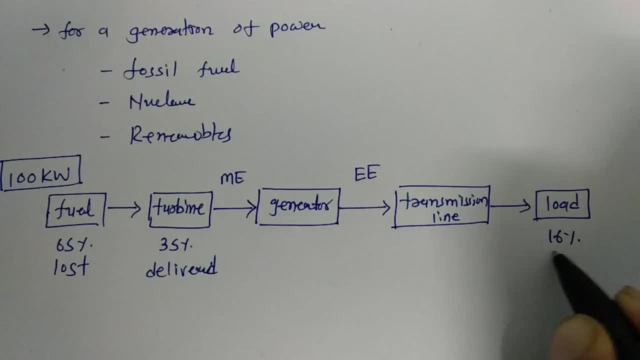 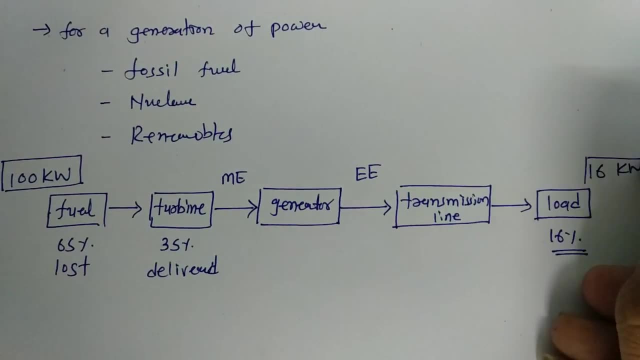 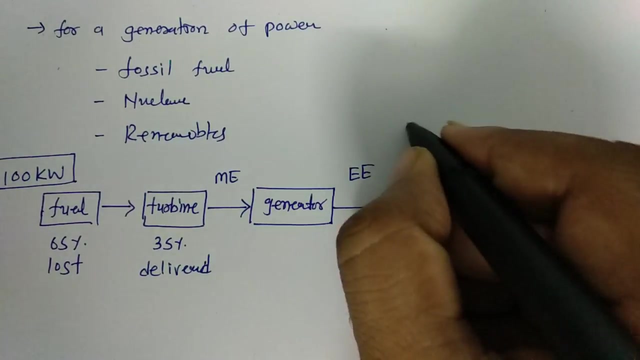 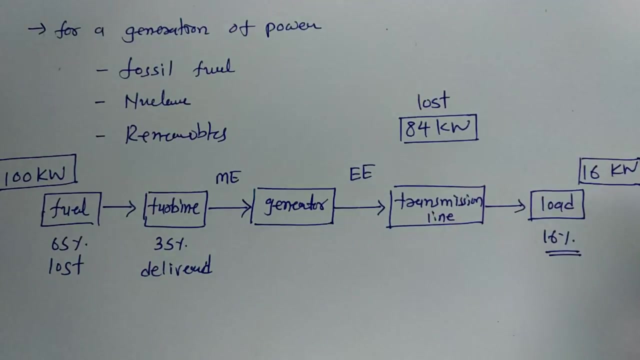 And at the end The power which is what delivered. that is 16 percentage only. So at the load side one can see 16 kilowatt power that is getting delivered. So during this entire process, 84 kilowatt power that is lost. 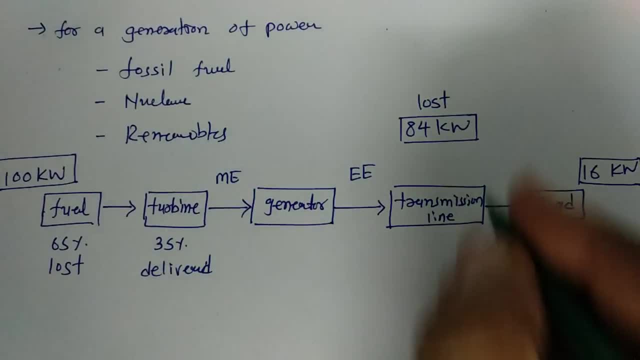 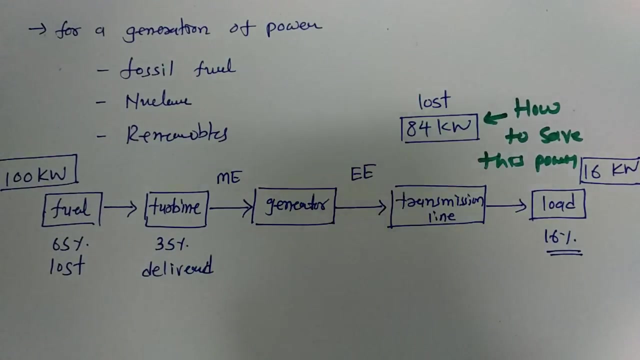 So now how we can save this power, How to save this power, So how many things are possible. Now one can understand here: we have power electronics rule at generator side, at transmission lines side, as well as at the load side. if we can optimize this power electronics in 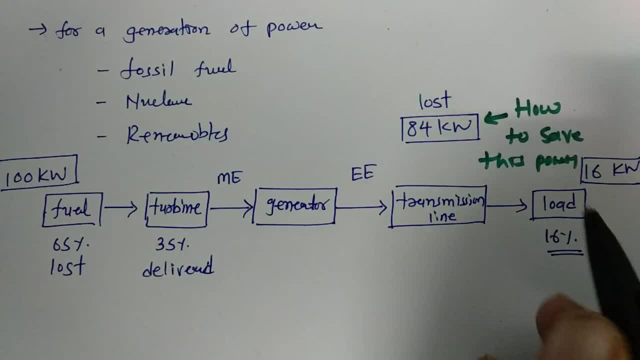 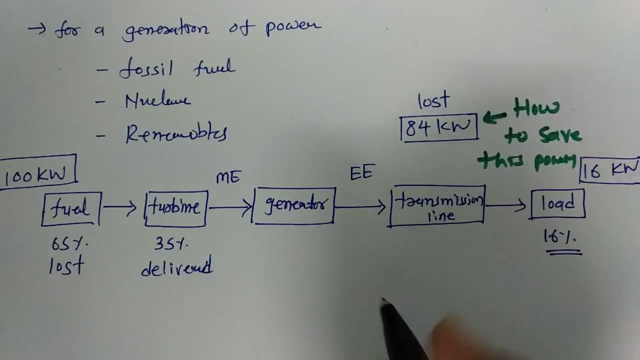 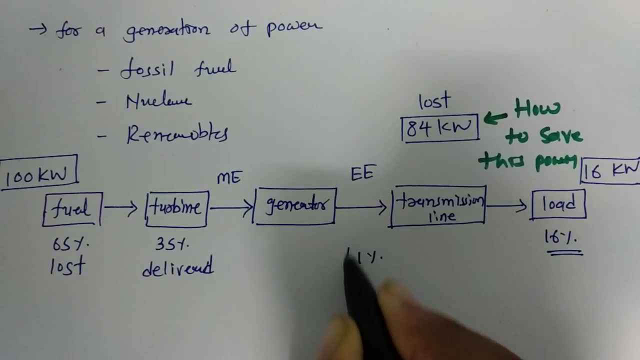 that case It is possible. one can save fractional amount of power which is getting lost over here. So, for example, if I say one is able to use electronics in a better way and if even you improve complete process by 1%, If somebody is able to improve a process by 1%. 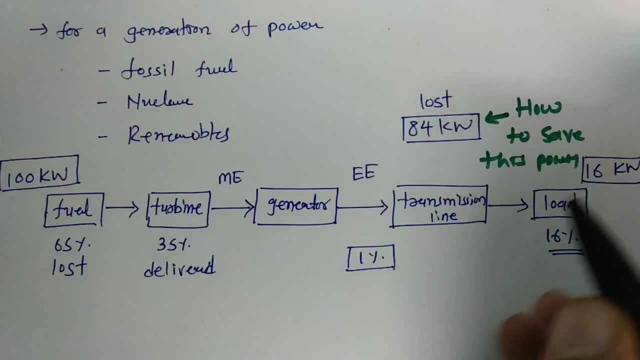 In that case, for 1 kilowatt. one can be able to improve power delivered to the load by 1 kilowatt, But if we see the amount of power which is being used by different countries, then this power that is there in terms of gigawatt. 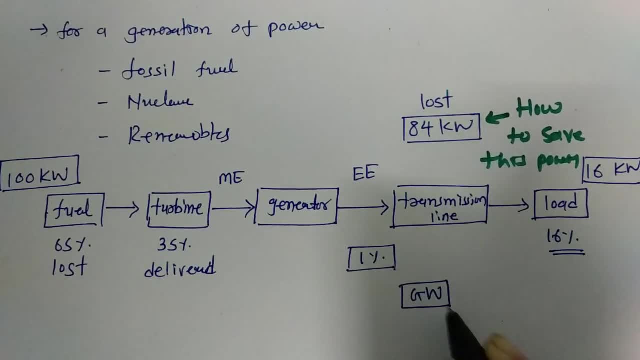 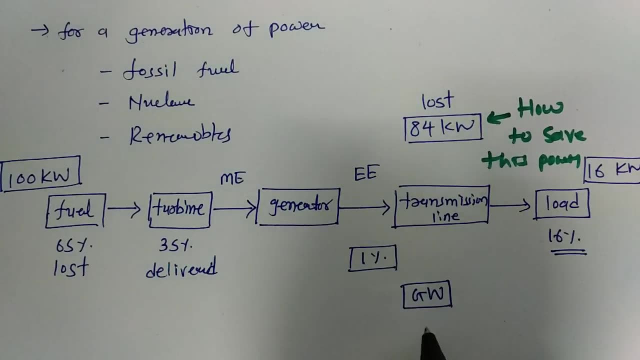 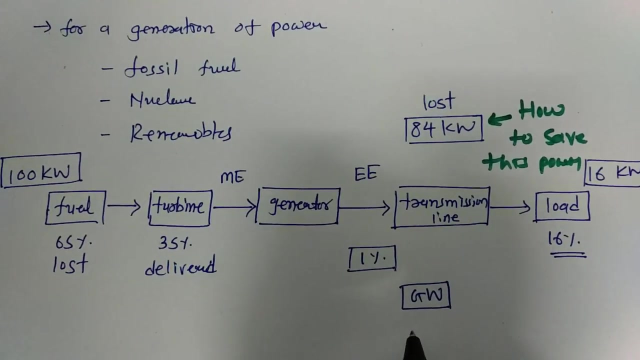 It is there in terms of gigawatt. So even if we improve this power delivered to the load By only By only one percentage, one can be able to improve power saving in terms of gigawatts. So see, this is how one can improve a technology which is existing by using power electronics. 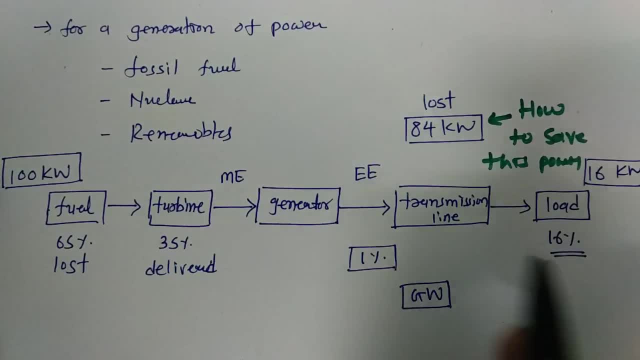 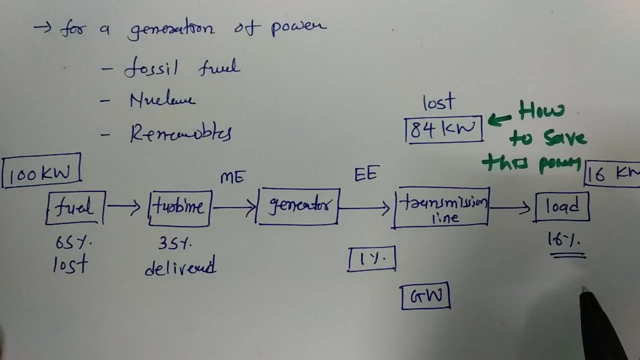 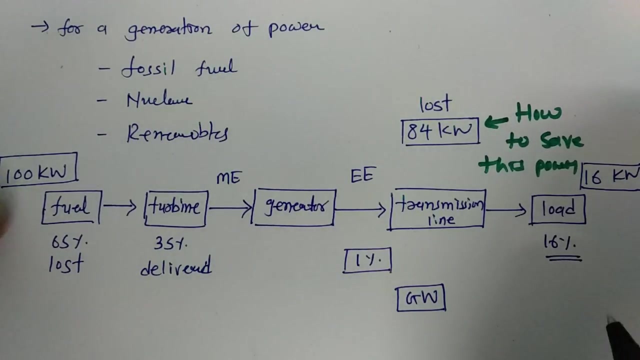 So where in this complete process there are different types of circuits, which is what we are using it in our, in our usual system, Like AC to AC converter, AC to DC converter, DC to AC converter, and when we are using all those things, at that time always there is what somewhat loss which is happening during the processes, and to optimize that system, all we can do is we can have such system which is having higher efficiency. 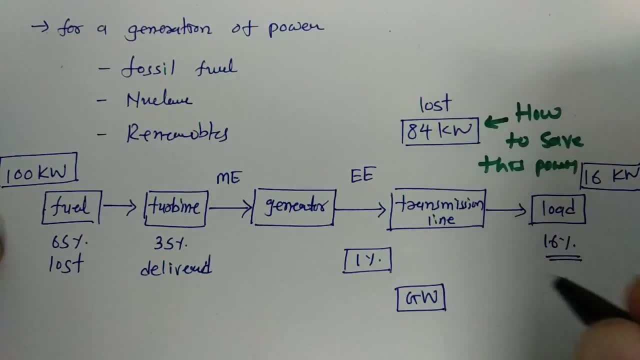 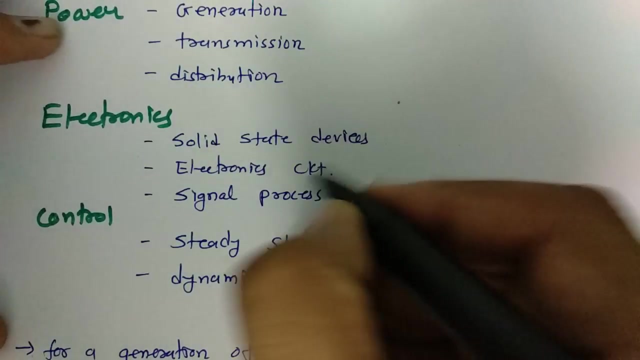 So by studying this power electronics subject, One can be able to optimize that This is the existing system and this is what the people were been doing by studying this power electronics. So this is what even we are delivered to do it with this playlist, where I will begin this complete power electronics with. first. I will be beginning this power electronics with solid state devices. 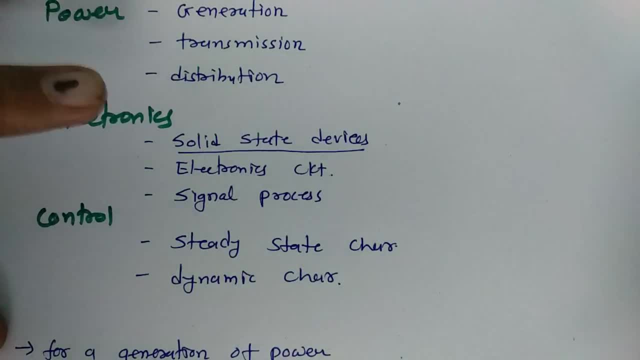 So this is what I will begin with with this playlist, where I will be explaining some small solid devices like SCR, IGBT, DIAC, TRIAC, SUV. So there are so many devices, which is what there in industrial applications, that I will be going to explain over here in this playlist. 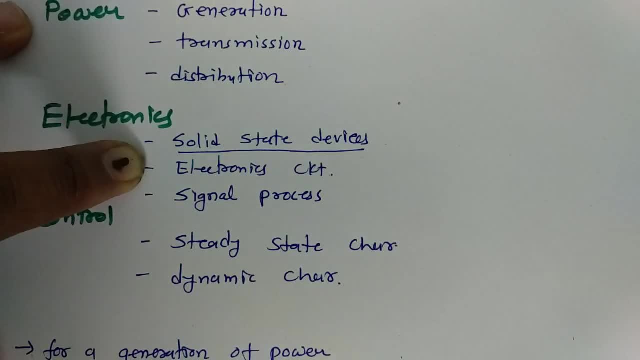 Then we'll see some electronic circuit, which is what very useful in so many aspects, where one can identify how we can have smart use of current system which is existing, and even I'll be going to explain some signal processes at high power, and then I'll explain some. 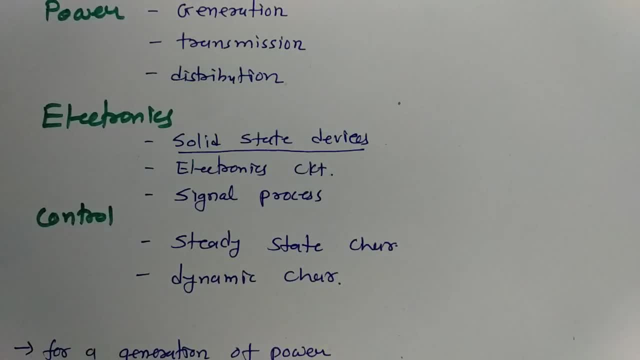 applications, which is very useful in power electronics. So ultimately, this playlist is all about basic understanding of power electronics. So this will be very useful for beginners. So stay tuned with my playlist. In next few videos we'll be going to knowing like see how things are happening in power electronics. 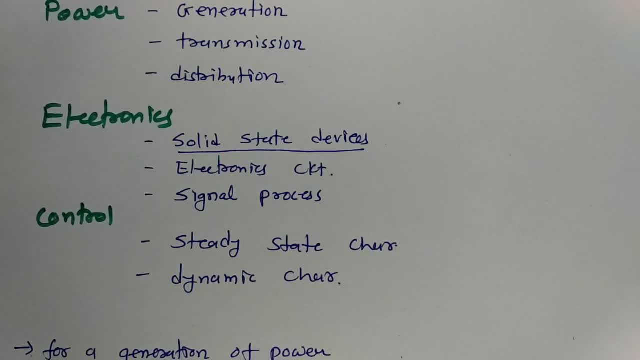 how many devices are there, how to utilize those devices. So my next session that will be there, based on working of SCR: internal structure of SCR- operation of SCR. Thank you so much for watching this video And if you have any query regarding this subject, you just give your advice. you write. 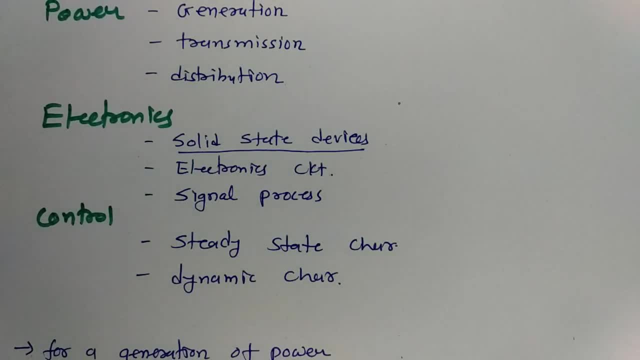 down your topic suggestion in comment so that I can be able to make out videos based on what is very useful to students in their study. So I'm waiting for your comments. You just write down comments in link below so that we can have a discussion even. Thank you. Thank you so much for watching this video.